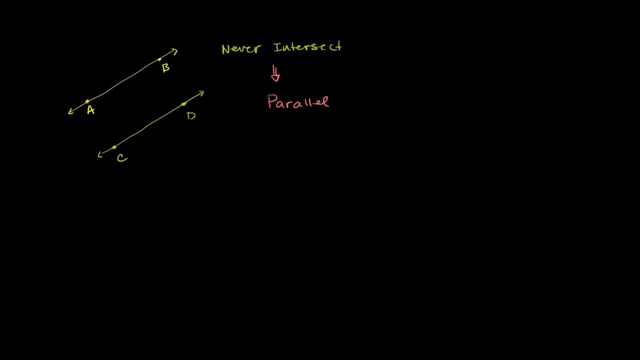 relate to parallel lines. So right over here we have these two parallel lines. We can say that line AB is parallel to line CD. Sometimes you'll see it specified on geometric drawings like this. They'll put a little arrow here To show that these two lines are parallel. 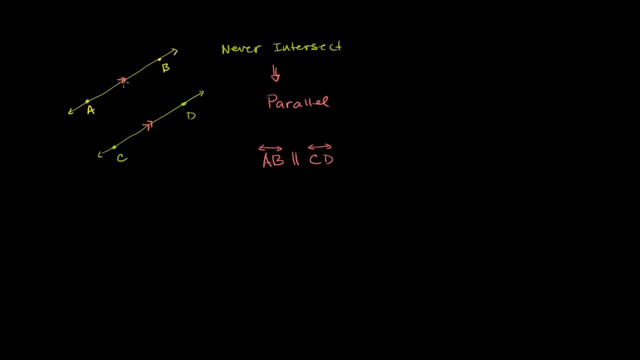 And if you've already used the single arrow, they might put a double arrow to show that this line is parallel to that line right over there. Now, with that out of the way, what I want to do is draw a line that intersects both of these parallel lines. 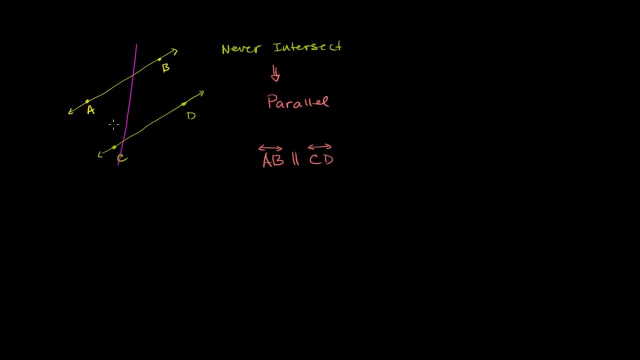 So here's a line that intersects both of them. Let me draw a little bit neater than that. So let me draw that line right over there And I'll just call that line. Well, actually I'll do some points over here. 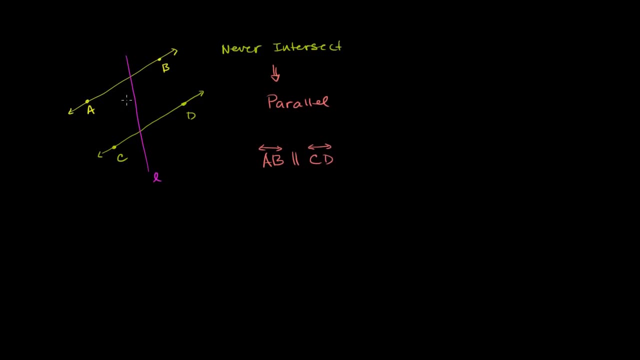 Well, I'll just call that line L And this line, this line that intersects both of these parallel lines. we call that a transversal. This is a transversal line. It is transversing both of these parallel lines. 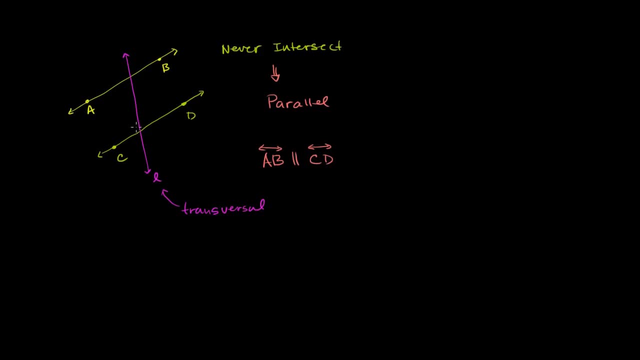 This is a transversal, And what I want to think about is the angles that are formed and how they relate to each other, the angles that are formed at the intersection between this transversal line and the two parallel lines. So we could first of all start off. 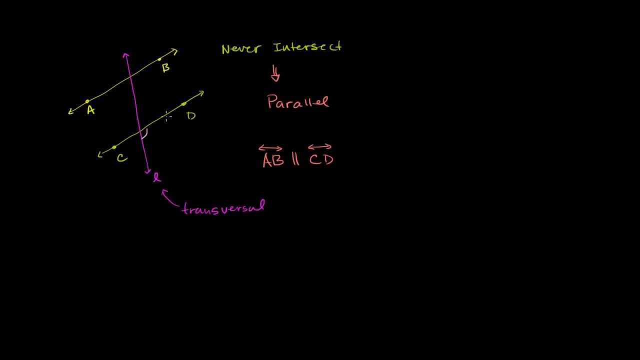 with this angle right over here, that angle right over there, And we could call that angle: well, if we made some labels here, that would be D this point and then something else, But I'll just call it this angle right over here. 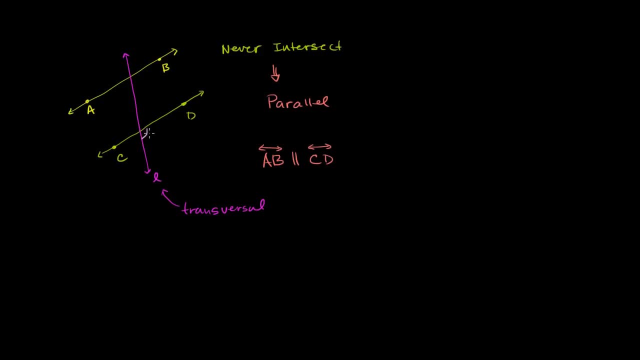 We know that that's going to be equal to its vertical angles. So this angle is vertical with that one. So it's going to be equal to that angle right over there. We also know that this angle right over here is going to be equal to the angle that. 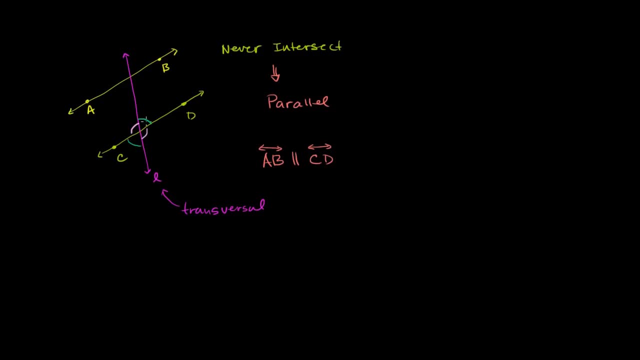 is at its vertical angle, or the angle that is opposite the intersection. So it's going to be equal to that, And sometimes you'll see it specified like this: We'll see a double angle, We'll see an angle mark, like that: 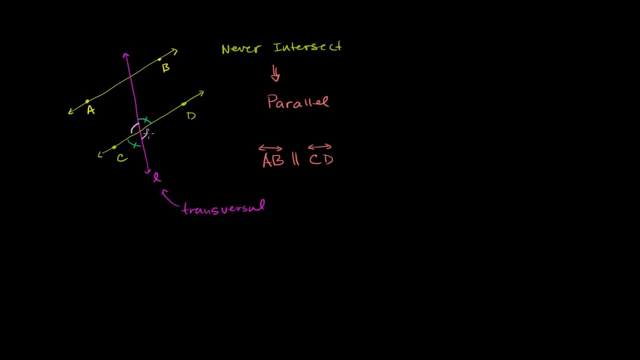 Or sometimes you'll see someone write this to show that these two are equal. and these two are equal right over here. Now, the other thing we know is we can do the exact same exercise up here- that these two are going to be equal to each other. 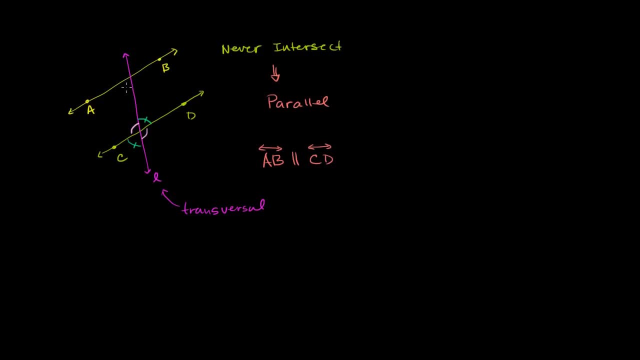 and these two are going to be equal to each other. They're all vertical angles. What's interesting here is thinking about the relationship between this angle right over here, the relationship between that angle right over there and this angle right up over here. 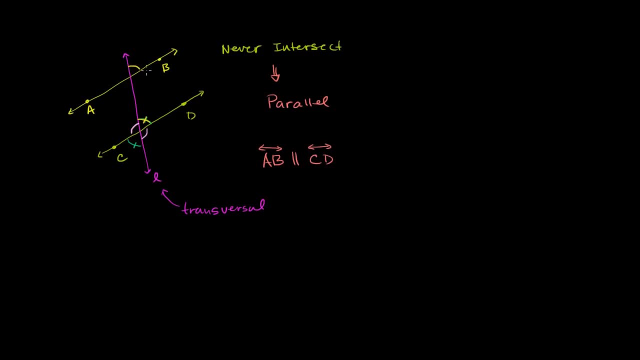 And if you just look at it, it is actually obvious what that relationship is, that they are going to be the same exact angle, That if you put a protractor here and measured it, you would get the exact same measure up here. And if I drew parallel lines, maybe I'll. 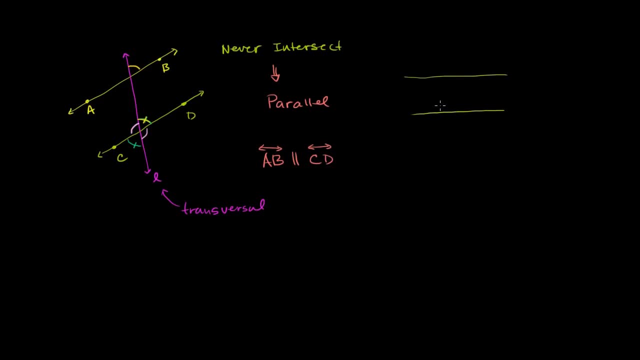 draw it straight left and right and it might be a little bit more obvious. So if I assume that these two lines are parallel and I have a transversal here, what I'm saying is that this angle is going to be the exact same measure. 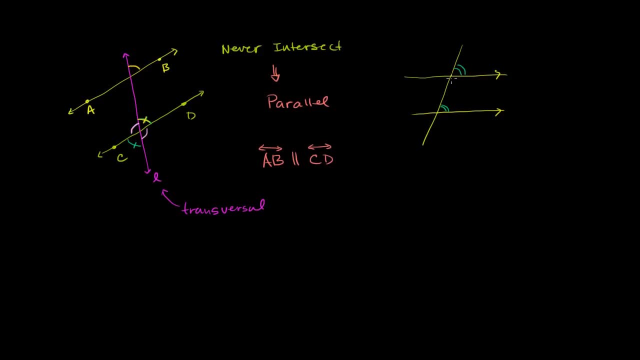 as that angle there And to visualize that, just to make it clear, just imagine tilting this line So it looks like it's the case over there. If you take the line like this and you look at it over here, it's clear that this is equal to this. 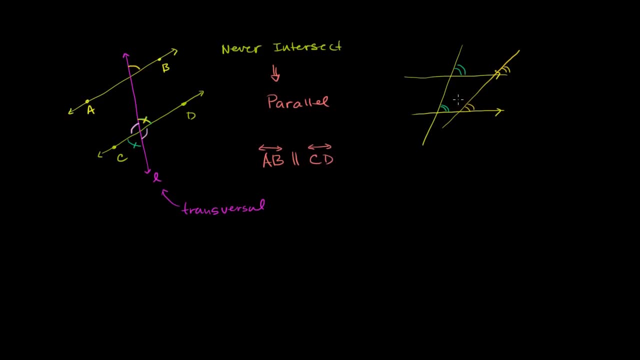 And there's actually no proof for this. This is one of those things that a mathematician would say is intuitively obvious: that if you look at it as you tilt this line, you would say that these angles are the same. Or think about putting a protractor here. 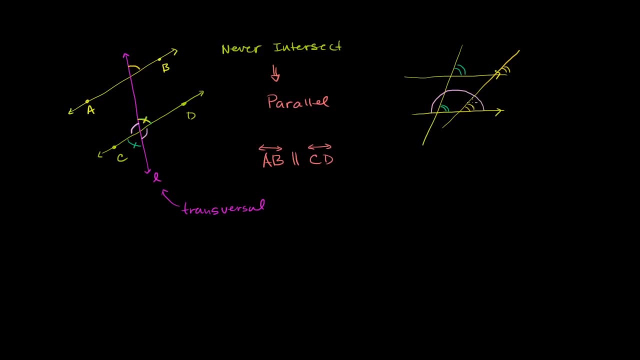 to actually measure these angles. If you put a protractor here, you'd have one side of the angle at the 0 degree and the other side would specify that point. And if you put the protractor over here, the exact same thing would happen. 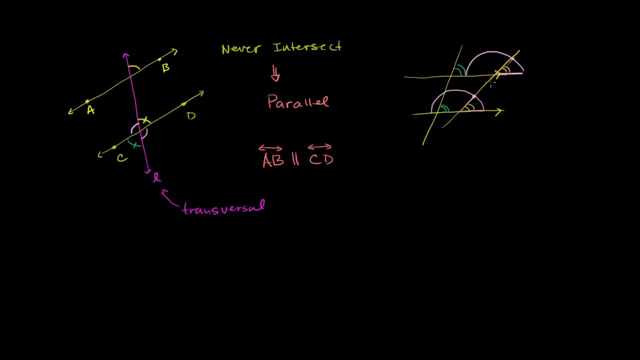 One side would be on this parallel line and the other side would point at the exact same point. So, given that we know that not only is this side equivalent to this side, it is also equivalent to this side over here, And that tells us that that's also equivalent to that side. 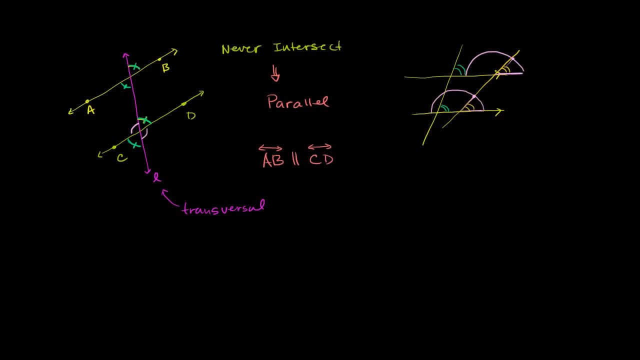 over there. So all of these things in green are equivalent And, by the same exact argument, this side right over here, or this angle, is going to have the same measure as this angle And that's going to be the same as this angle because they are opposite or they're vertical angles. 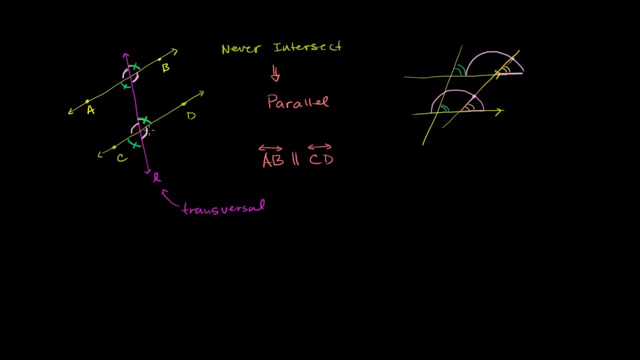 Now, the important thing to realize is just what we've deduced here: The vertical angles are equal, and the corresponding angles at the same points of intersection are also equal, And so- that's a new word that I'm introducing right over here- This angle and this angle are corresponding.